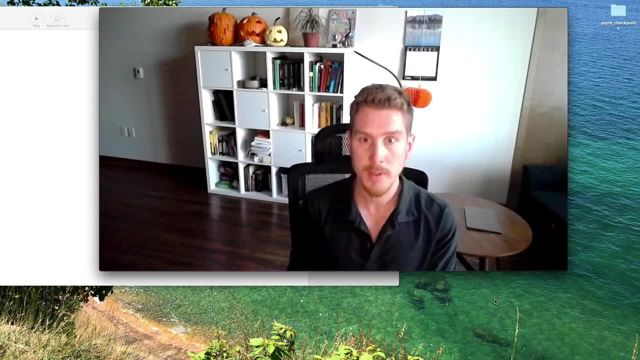 to a new topic, which is, I hope, exciting. So in this new series of lectures, which will be on model evaluation, we won't be introducing new machine learning classifiers or algorithms. we will be learning how to assess the algorithms that we talked about in the past, fairly So there. 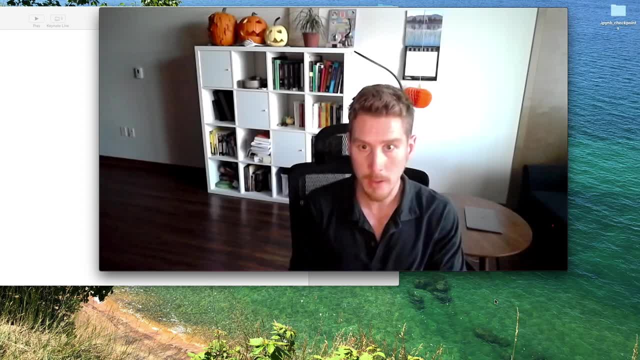 will be a series of lectures related to understanding underfitting and overfitting, how that's related to the bias and variance decomposition of a loss function, And then we will move on and take a look at cross validation methods that allow us to compare models fairly. 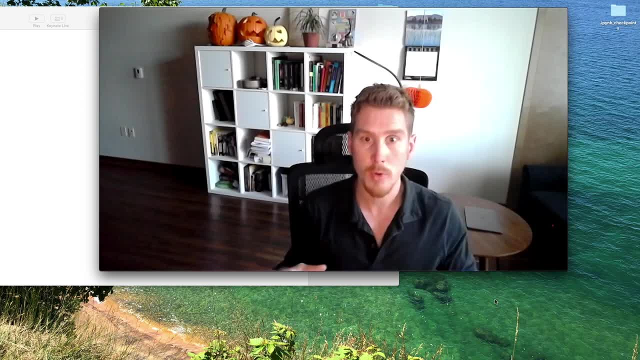 And then we will also later on talk about methods to compare machine learning algorithms to each other so that you can have an idea of what type of algorithm may perform good on a particular data set in terms of the generalization performance. So there's a fine grained, I would say, difference between 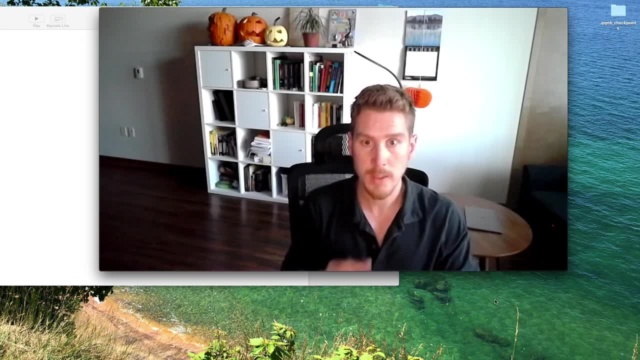 model selection, which basically is concerned with selecting a model that has been fit, versus selecting a good algorithm and machine learning algorithm, And we will discuss this in more detail. And with that, yeah, I would say, let's just get started with the introduction. 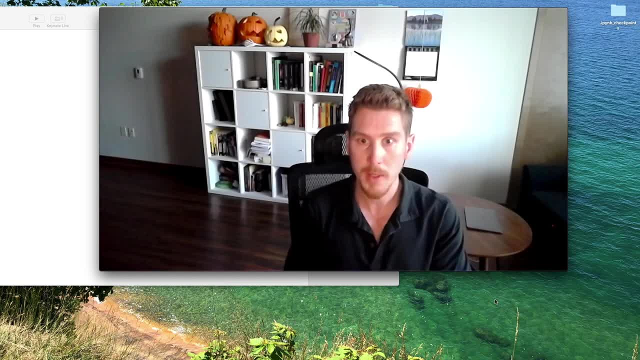 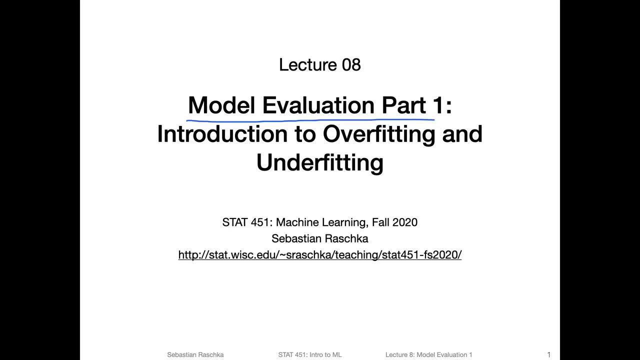 to model evaluation And we will continue from there. Yeah, we are about to start a very interesting journey into the topic of model evaluation. there will be plenty of topics to talk about And we will start gently by an introduction to overfitting and underfitting. However, before we start, just a brief overview where we are in this. 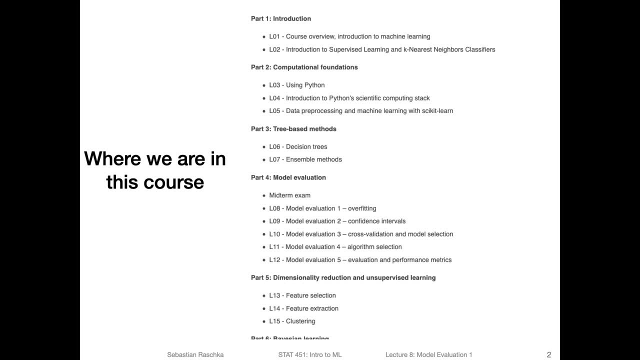 course. So this is probably trivial, but I think it's sometimes good to just check ourselves where we are, what we have covered and where we are heading. So, as you all know, we covered the introduction. we talked about the computational aspects like Python, NumPy, second learn. 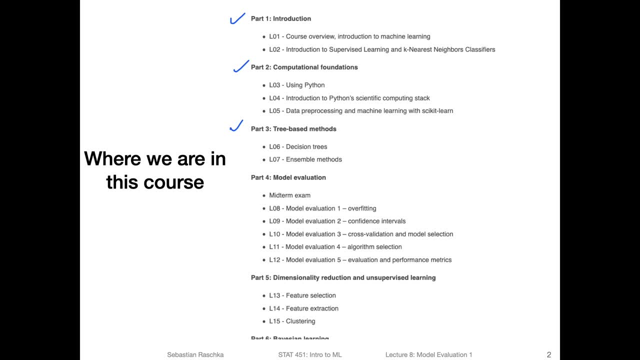 we talked about tree based methods And I remember there were some interesting questions, like our tree based methods still relevant because the algorithms we talked about there were pretty old. However, no, there are also some new algorithms, like the one I posted on Piazza about the online. 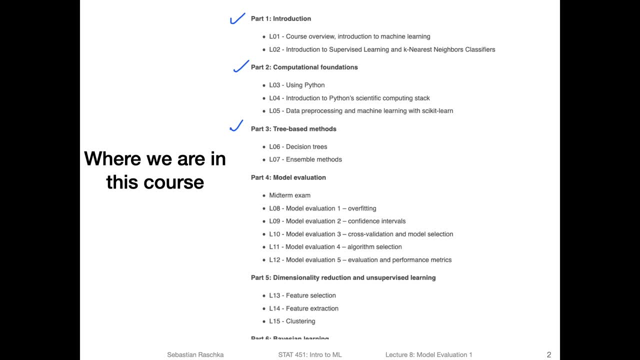 decision trees and so forth. The main answer to this question: are decision tree algorithms still relevant? The answer is yes, because there were these ensemble methods that we talked about, particularly boosting, gradient boosting and random forests, which are very popular still in industry. And then yeah, now. 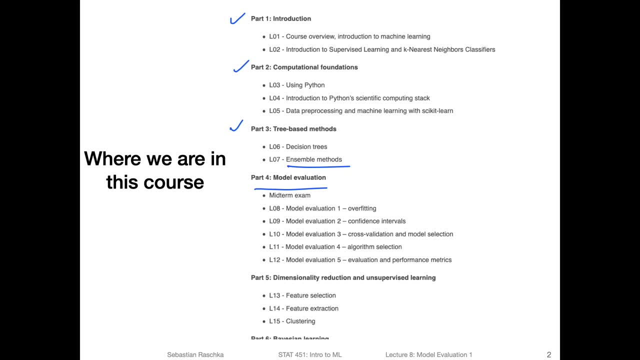 we are going to cover model evaluation. there will be several subtopics. on the topic of underfitting and overfitting, we will talk about confidence intervals, cross validation, model selection, algorithm, selection, evaluation and performance metrics, and so forth. And then, lastly, we will 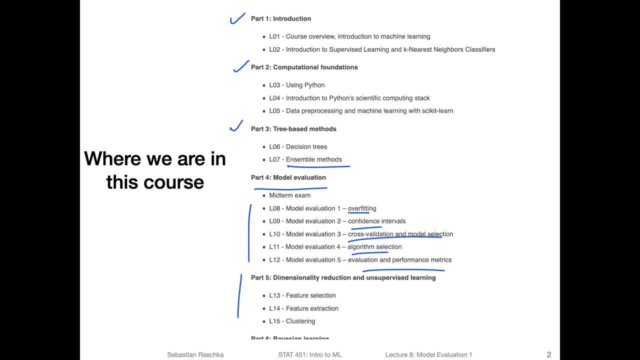 talk about dimensionality reduction and unsupervised learning once we finish the model evaluation lectures, But let's, let's focus on part four Now, before we go too far ahead talking about topics that we haven't covered yet. Yeah, but also to summarize the model evaluation. 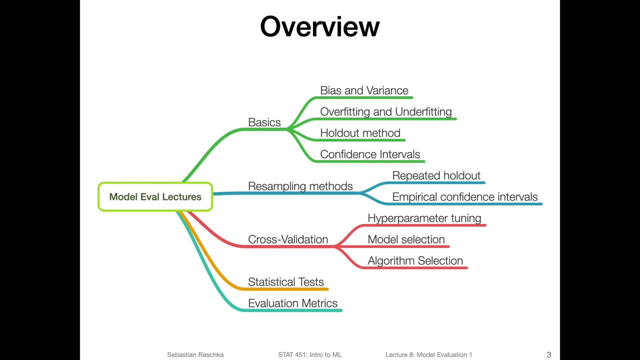 lectures there will be plenty of topics to talk about. So in this particular lecture, in lecture eight, we are going to talk about the bias and variance decomposition and how that relates to overfitting and underfitting. So that's lecture eight. that we are covering right now And then in the future lectures we will talk about. 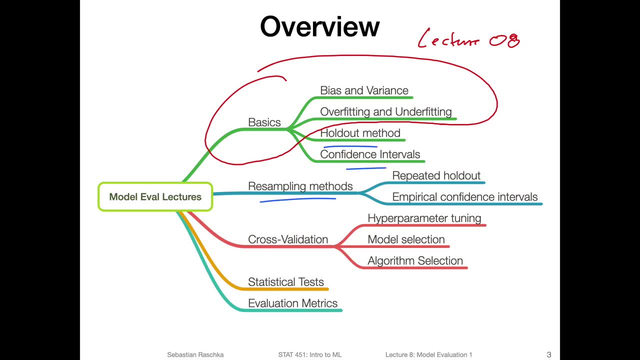 the holdout method confidence intervals. we'll talk about certain resampling methods, like the repeat repeated holdout method, how we make empirical confidence intervals using the bootstrap techniques. We talked a little bit more about cross validation and then we will talk a little bit more about cross validation- how we use cross validation for hyper parameter tuning. 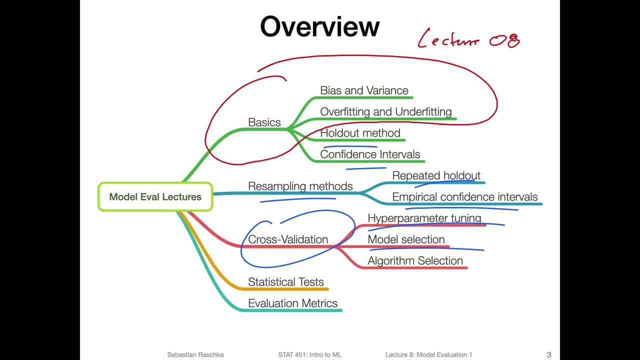 which is the topics related, closely related, to model selection, And then we will, lastly, also take a look at some techniques for algorithm selection that are based on cross validation, such as nested cross validation, And then, after that, we will talk about some statistical tests that we can use. 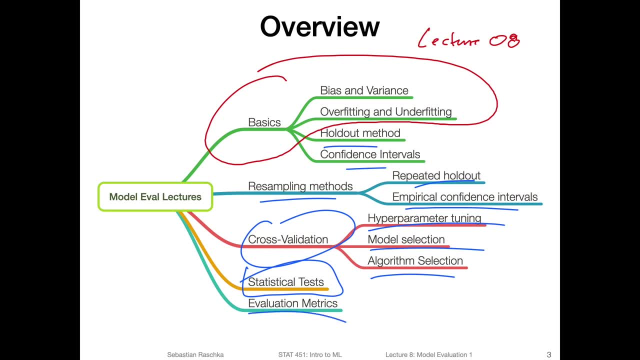 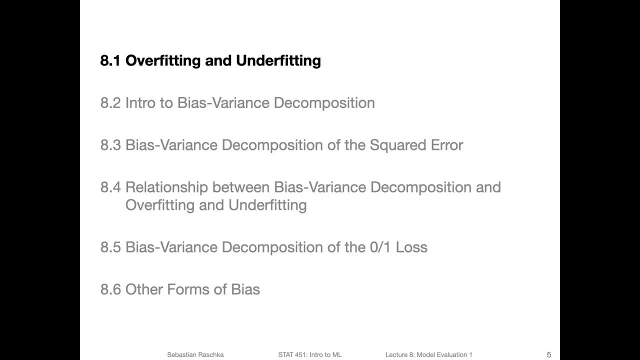 for comparing models and algorithms, And then we will also talk about evaluation metrics, for example the receiver operating characteristic under the curve and others. But yeah, now let's get started with this lecture, the introduction to overfitting and underfitting. 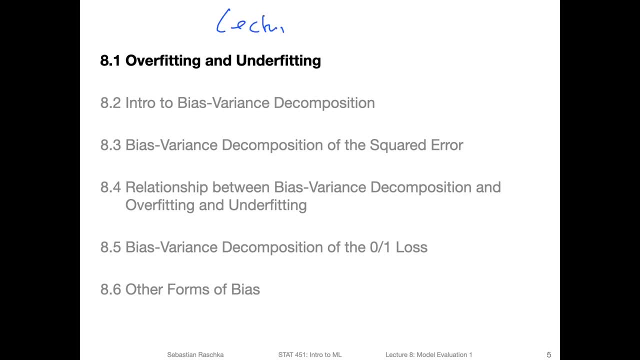 And I structured lecture eight into six subtopics. This time they will be way shorter than usual, because this is a relatively short lecture, especially compared to the ensemble method lecture that we covered last time, which was ridiculously long, but I thought it was kind. 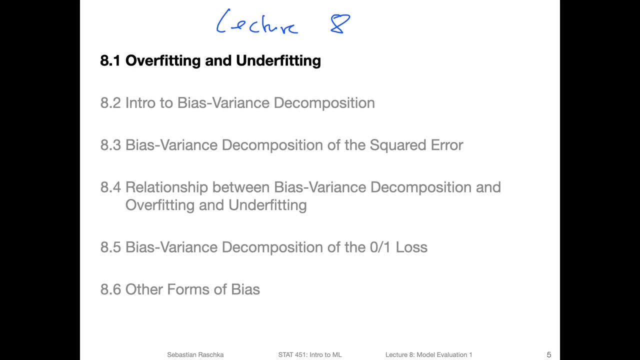 of necessary, because ensemble methods are quite important topic in practice. So I wanted to give at least some time and focus because, yeah, you will likely encounter them in practice at some point. So, yeah, we will cover or we will just briefly introduce overfitting and underfitting. 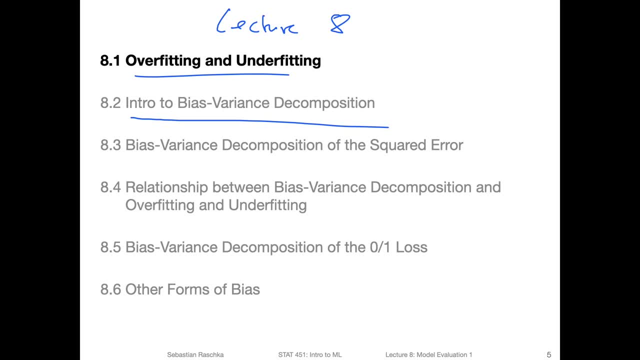 And then we will introduce the bias and variance decomposition. we will actually will form a bias variance decomposition of the squared error loss And then we will, after we saw how that works, we will talk about how that's related to overfitting and underfitting. So what's the relationship between? 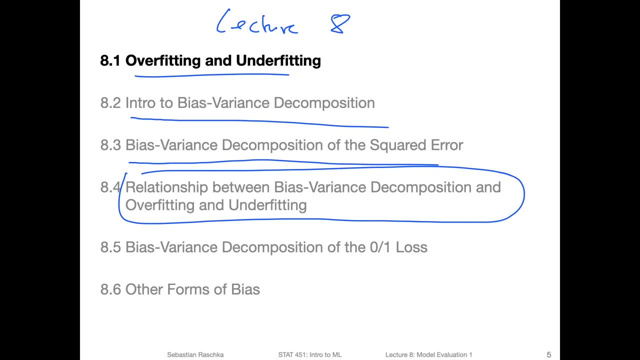 the bias variance decomposition and overfitting and underfitting, And then we will also do the bias variance decomposition of the 01 loss, because this would be more like relevant for regression And this would be more like the case for classification. I mean the basic understanding or 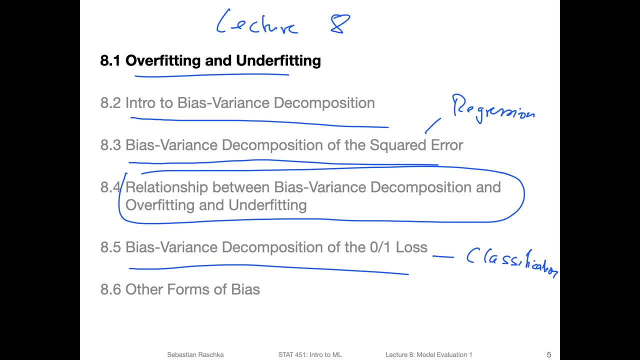 interpretation of that is the same. I mean, the main point is: how does it relate to overfitting and underfitting? but I think it's still interesting to look at the bias variance decomposition in the context of the 01 loss too. 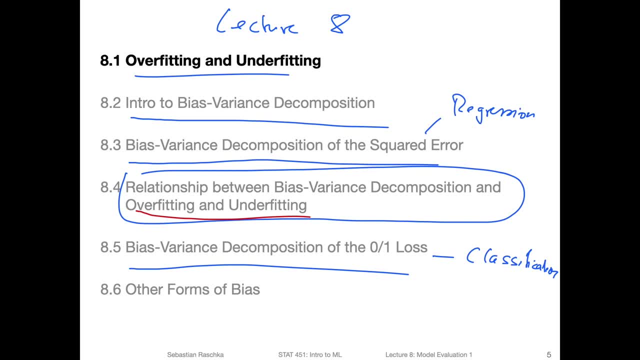 because that's a little bit trickier and it relates more closely to the classification problems that we more often work with in machine learning. And then, just briefly to wrap up this lecture, we will briefly also talk about different types of biases in machine learning, beyond just the statistical bias. 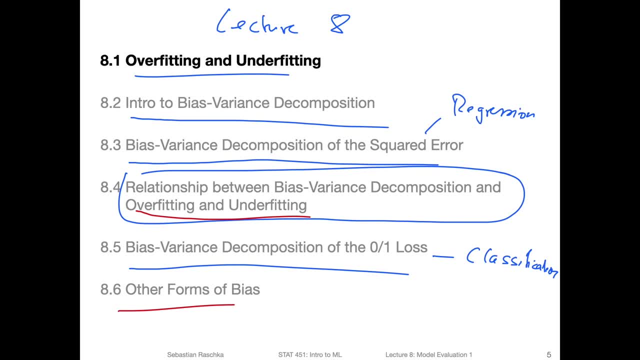 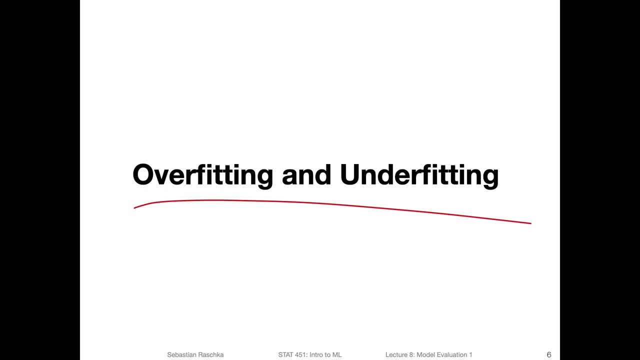 or the bias, when we decompose the loss function here. Okay, let's get started, then, with overfitting, Overfitting and underfitting. what is overfitting and what is underfitting, And in order to talk about this, let's think of 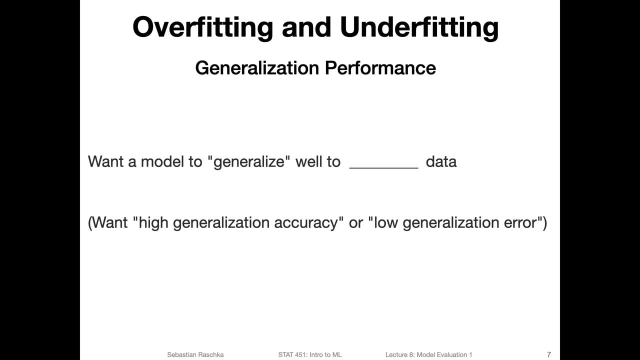 the main goal that we care about in machine learning. Of course there are many main goals like solving a particular problem, But from a general perspective the main goal is in machine learning to develop an a model- could be a regression or classification model- that has a good generalization performance. 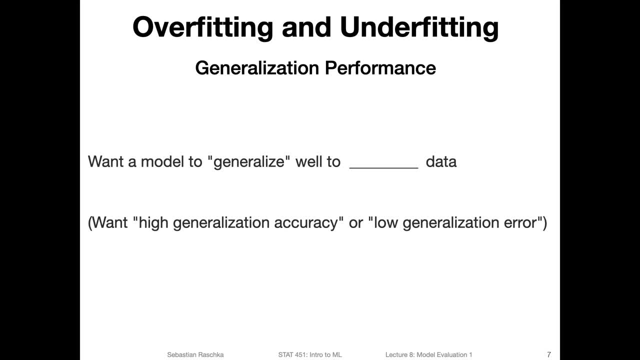 That means that once it's trained on some data set that it generalizes well to some new data that comes from the same distribution. The new data is usually some unseen data on the test set data. if we talk about model evaluation, because the test that is usually the data set of unseen data points that 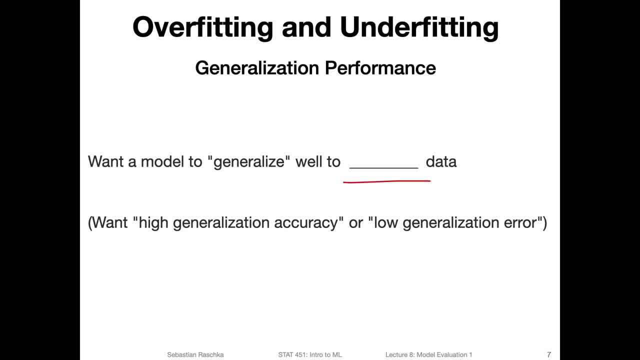 we use for evaluating our model. So I have this little blank here also to remind myself to ask you questions, sometimes about topics I'm talking about in the lecture, beyond just asking you in the quiz, Because I think sometimes it's helpful Also just to pause the. 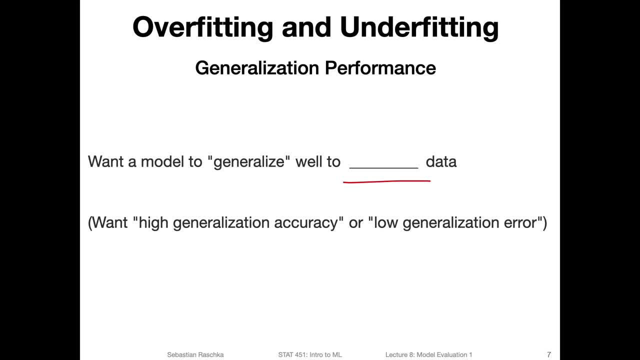 video and also think about what you think, what your opinion is, before I share my opinion here. So here I'm basically asking: what do we really want in machine learning? So what? what do we want from a model? So we want a model to generalize, well, to. 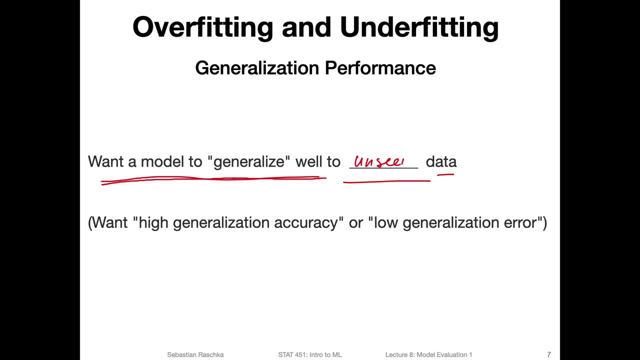 what type of data? so I would put here unseen data, because that's that's really what we want. We want our model to perform well on unseen data. of course, there are limits. it can't be just any type of data data. So if you train a model to perform, I don't know, stock 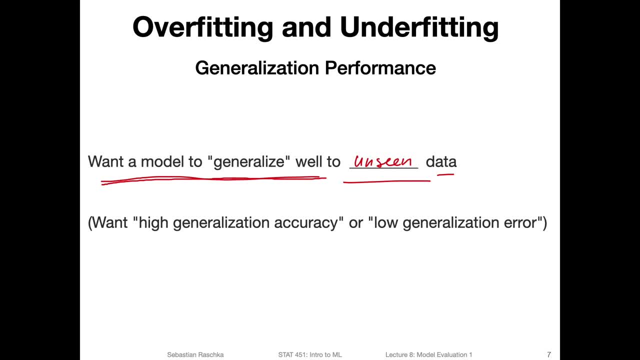 market predictions. you can't expect the model to perform well on a data set of cat and doc images, of course, So the data has to come from the same distribution as the training set data, of course. But yeah, what we really care about is the 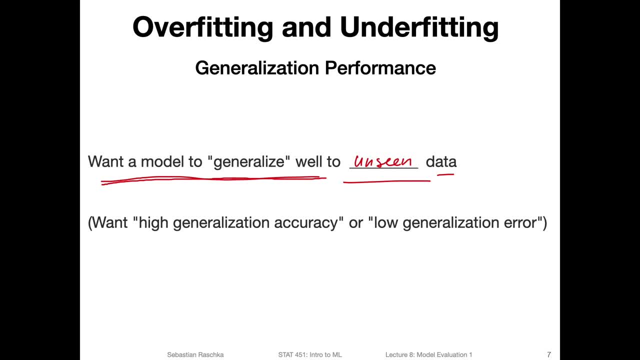 unseen data that our model generalizes well to unseen data. Of course we also care about performance on the test set data, But this is more like something we care about. when we write academic papers and we want to show how awesome our model is, then we also care about that the model performs. 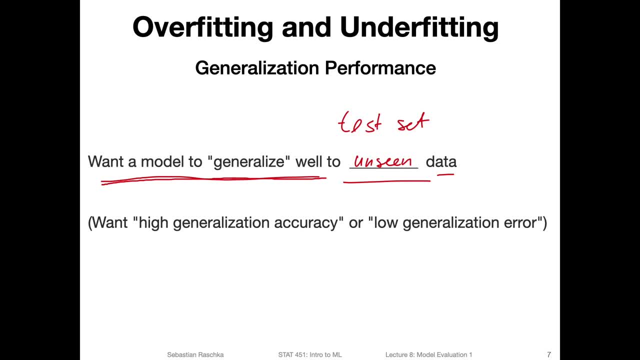 well on the test set. But usually I mean, the test set is just a proxy, It's just a method for estimating the generalization performance on unseen data. So what we really want is we want a high generalization accuracy. Or if we speak of the error, it's: 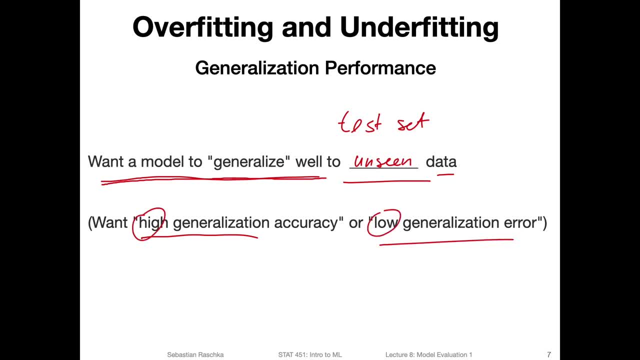 like inverted. So instead of high we have the low generalization error. So we want to have a good generalization performance, which means high generalization accuracy or low generalization error, which are usually equivalent because the accuracy is defined as one minus the error. when we talk about 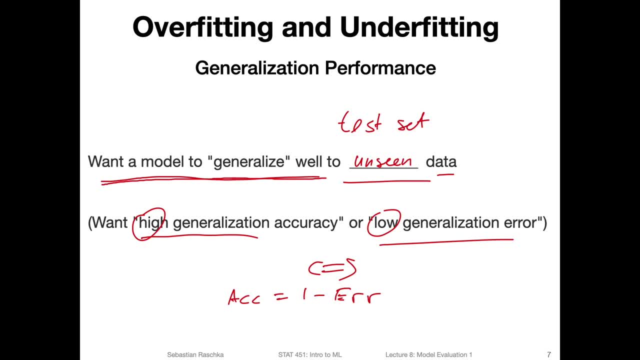 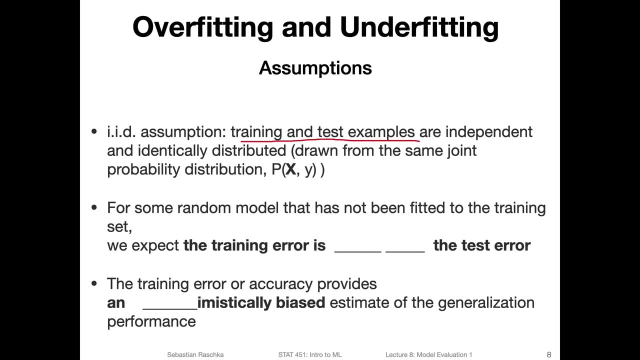 classification accuracy or misclassification error. Yeah, when we talk about the generalization error, we usually make assumptions, So we assume that the training and the test examples are independent. So we are here for the next couple of lectures, assuming independent. 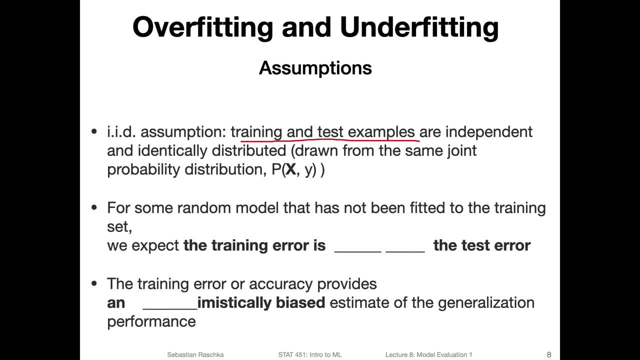 Okay, data points, not time series data. time series data is a bit tricky and beyond the scope of this course. So here we are explicitly looking at independent examples And we also assume that they are identically distributed, So they are drawn from the same joint probability distribution. So we have the 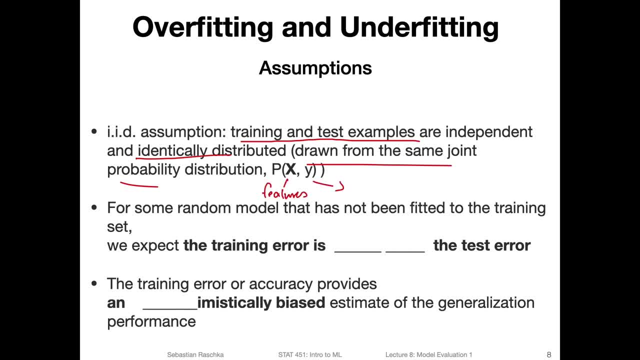 features and the labels or targets, So the joint distribution of these. So now another question for you: for some random model that has not been fitted or fit- we can say fitted or fit to the training set. we expect that the training error is smaller than larger than the test error. what do you? 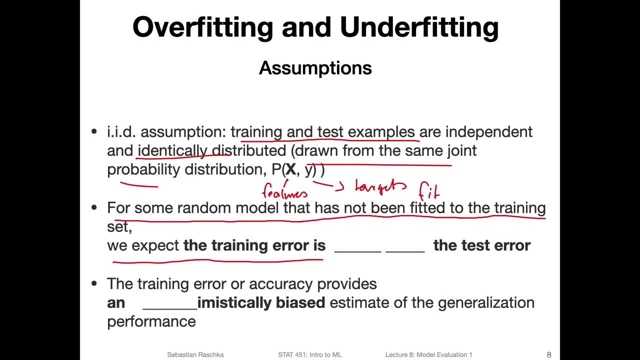 think, should the training error be larger or smaller than a test error? What would you expect usually in practice? So for a random model that has not been fitted to the training set, what I would expect is that the training error is approximately similar to the tested error, because if we don't fit the model, 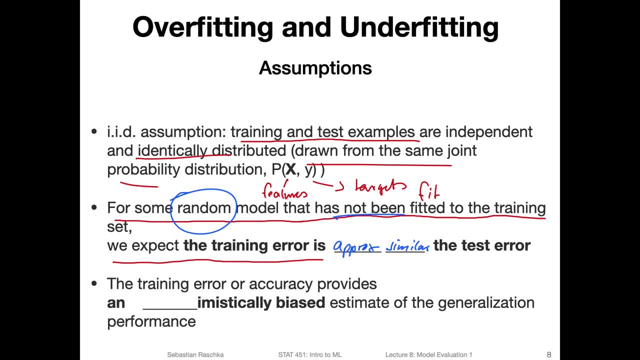 then yeah, usually no overfitting can occur, right? So in this case I expect the training order to be similarly large as the tested error For a model, though, that has been fitted to the training set. So for some model that has been fit or fitted to the training. 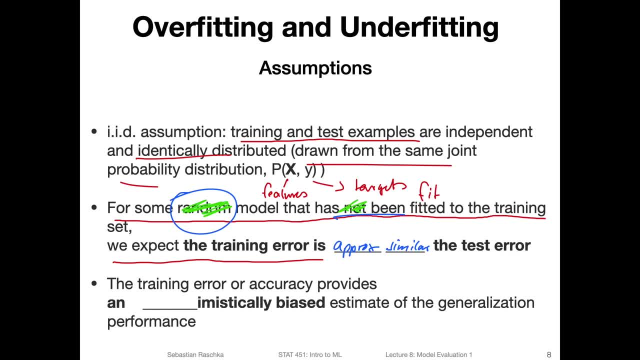 set, I would expect that the training error is larger than the tested error. That is because of overfitting And, in general, the training error or the training accuracy provides an optimistically or pessimistically biased estimate of the generalization performance. what do you think? So in this case, it would be an 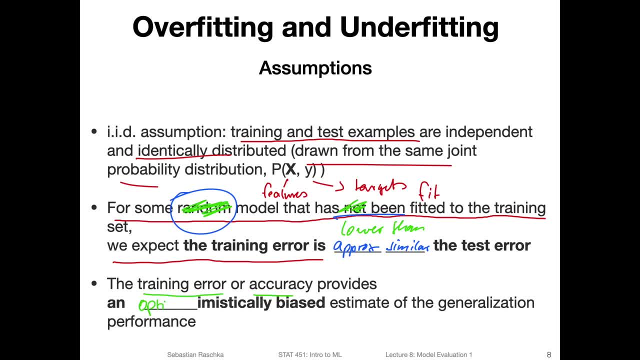 optimistically biased estimate of the generalization performance. And that is, yeah, just to the fact that the model has seen the training data and it has learned to perform well on this training data, because minimizing the loss on the training data kind of implies that we learn from this. 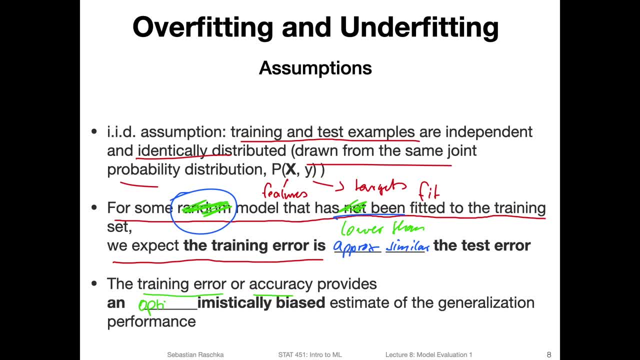 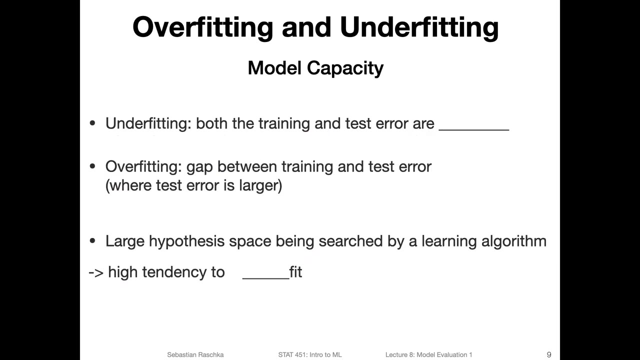 particular data set And sometimes this avoid. and sometimes this involves also fitting the model too closely to noise in the data, which usually leads to an optimistic estimate of the performance. So, for example, in practice we may observe that the training set accuracy is higher than the tested accuracy. So for 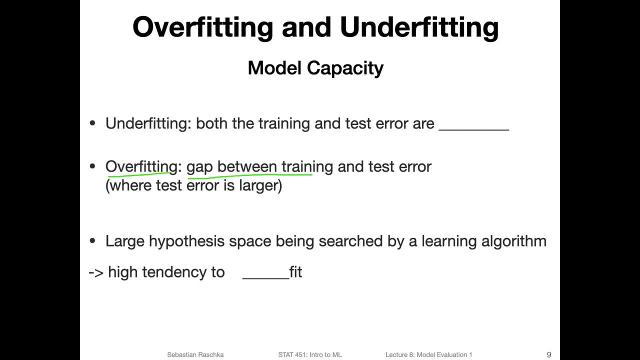 overfitting. what we often see is that there's a gap between the training and the test error, where the test error is larger And similarly the test accuracy is lower. Now, this is all fitting. what about underfitting? So how do we usually tell whether? 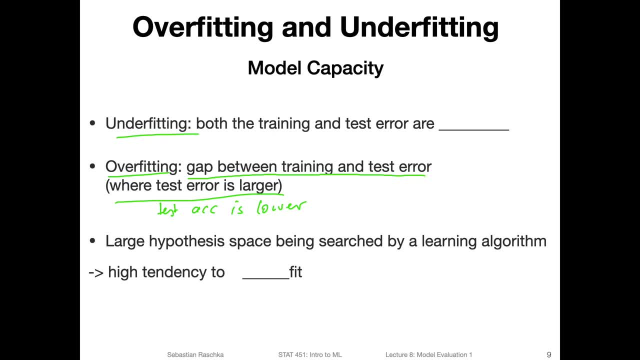 a model is underfitting the data set, So that means that it's usually not, I would say, strong enough or capable enough of capturing the patterns in the data that help with making good predictions. So in this case, when we are underfitting both the training and the test, error, 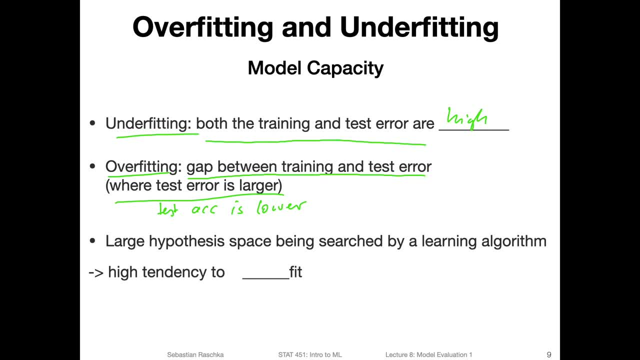 are high because the model, if it's underfitting, it's not really able to perform or extract useful information from the data Now related to the topic of hypotheses spaces. So a hypothesis space is the space that the algorithm, the machine learning, 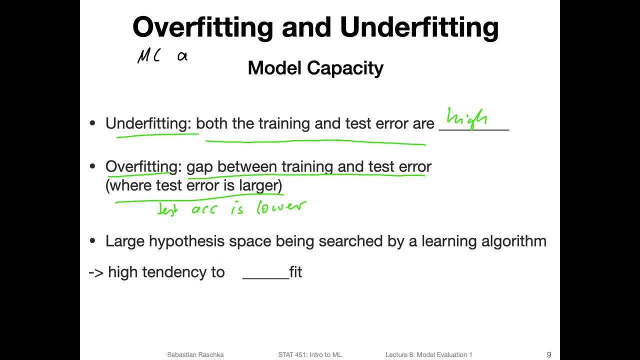 algorithm has access to. So say, we have a machine learning algorithm And the machine learning algorithm, even if we have the same data set, can produce many different models. So there are many possibilities for models that it may may produce, and that is related to what hyper parameters we choose. So there, 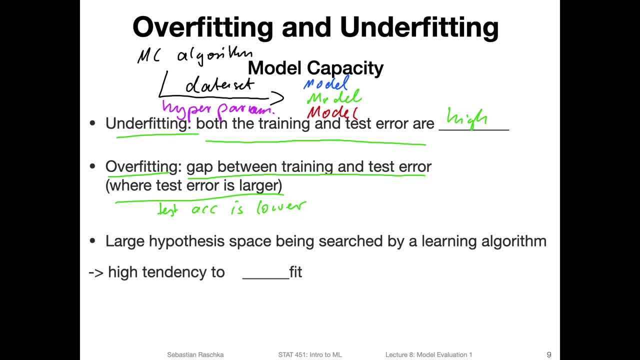 are many hyper parameter settings that we can choose and each hyper parameter setting, even if we don't change the data set, would result in the same model. Now also think about different training set samples from the same population. So if we have different data sets and consider that there are multiple, 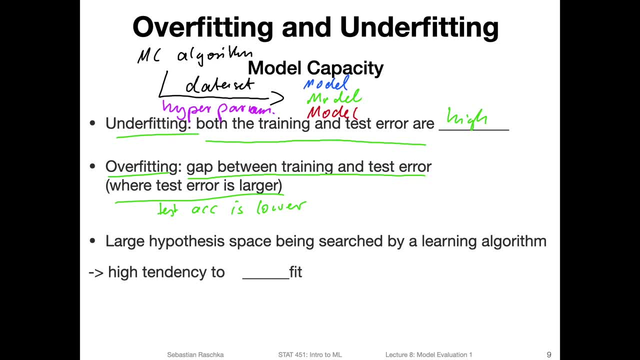 hyper parameter settings, then we could choose there as a large number of different models That could be the result of applying a machine learning algorithm And on this whole thing could be considered as a hypothesis space, where you think of a model as the hypothesis, the prediction hypothesis, And the larger the 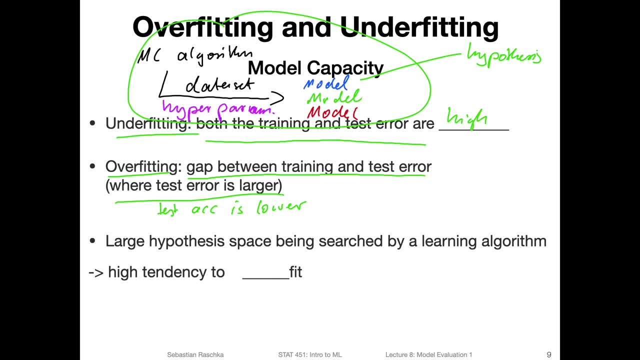 hypothesis space is so usually the more complicated the data set and the more hyper parameter options and machine learning algorithm has, the larger the hypothesis space that is being searched is. And the larger the hypothesis space is, the higher the tendency to over fit the data set. 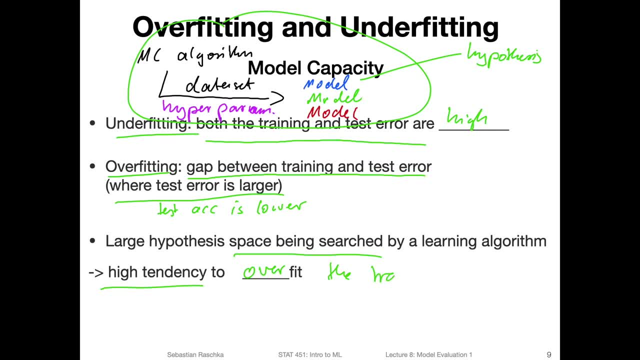 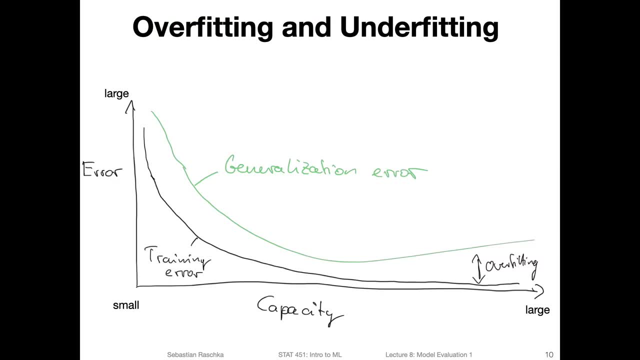 the training data set. Here's a brief sketch of the problem. It's just a sketch I made by hand And this should also illustrate that this is just an approximation. It's not like based on some real data, because that would be tricky, it It? 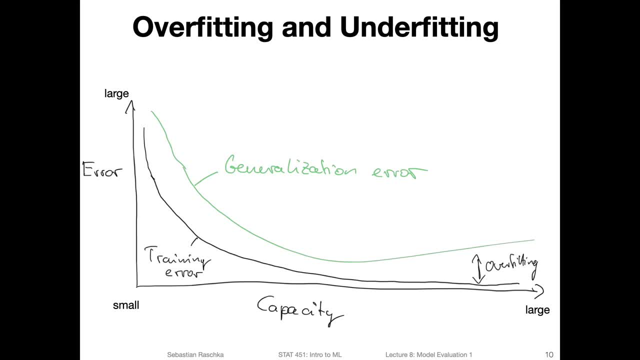 really depends on the algorithm and the type of data set. But here I'm just trying to capture the general relationship between the training set error and the generalization error. So here on the y axis I have just some measure of the error though. 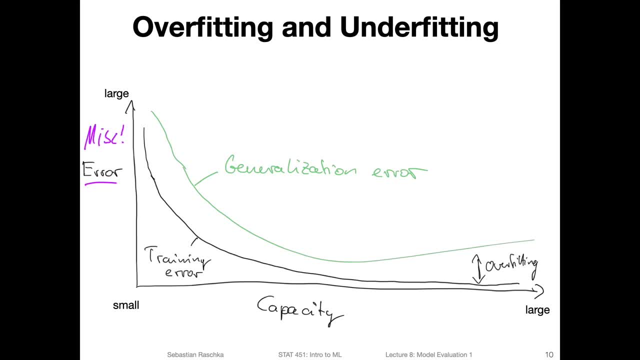 think of the misclassification error that could be small to large, And here I have the capacity of the model. So capacity is a little bit of a tricky term. the term capacity. it's kind of sometimes related to VC dimension, But in this course we are not going to talk about. 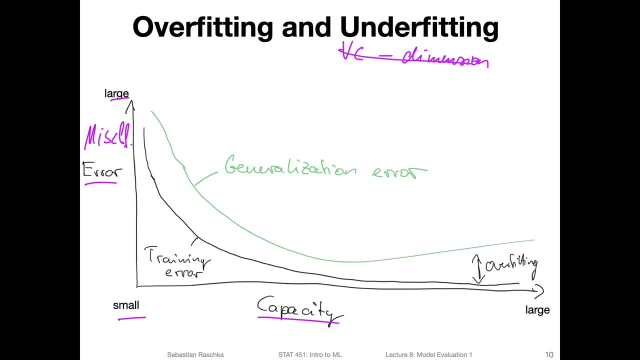 VC dimensions. it's a little bit too too much like out of the scope of this course because it would require more like background in machine learning theory. Yeah, but the intuition is that capacity is related to the number of parameters in the 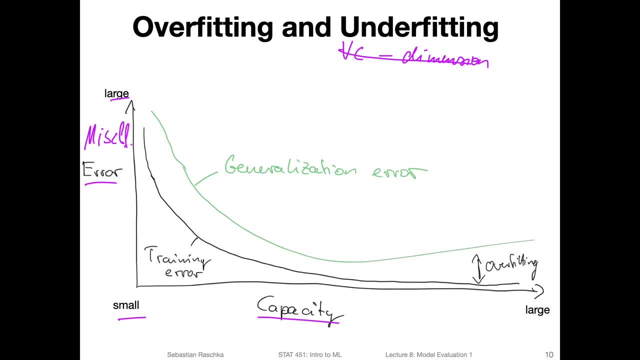 model Now again. the second issue is that in this class so far we talked mostly about non parametric models, but the same concept applies. So capacity really means how, how well the model is able to fit the data set. So a small or low. 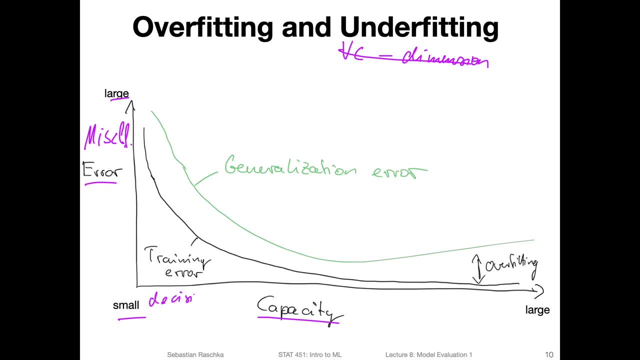 capacity model would be, for example, a decision tree stump, and a high capacity or large capacity model would be deep decision tree, because a deep decision tree has many more decisions. it's way more complex. So you can also think of capacity as maybe complexity of the model. So how well can 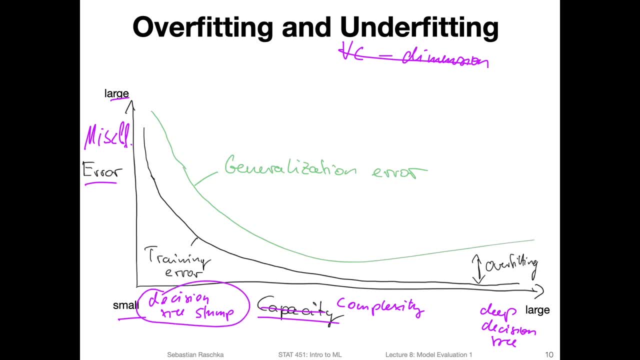 the model fit the training data set. So a decision tree stump cannot really fit the data very well because it's too simple. It can only make one split of the training data, So it can't really overfit so much. So in this case low capacity model is. 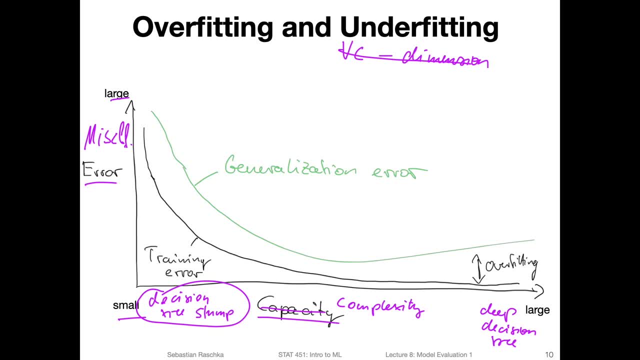 usually not overfitting. However, recall that a decision- tree stump- is so simple, yeah, that it doesn't fit the training set very well, which will then eventually lead to a high training error. So here this is the training error. So it's very 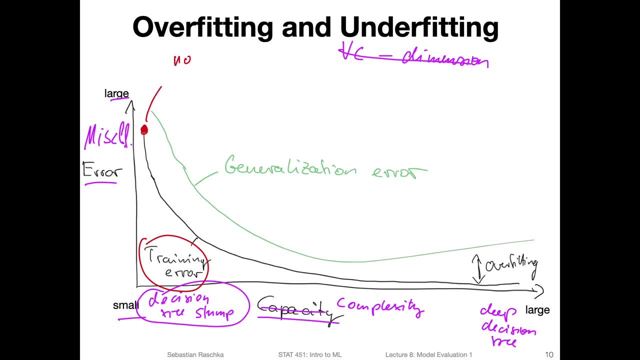 simple model, even maybe the one node- decision tree node- that we talked about in the context of gradient boosting. when we start the gradient boosting algorithm, it would be a case where we have a very large training error because the model is way too simple to fit the data set Well. 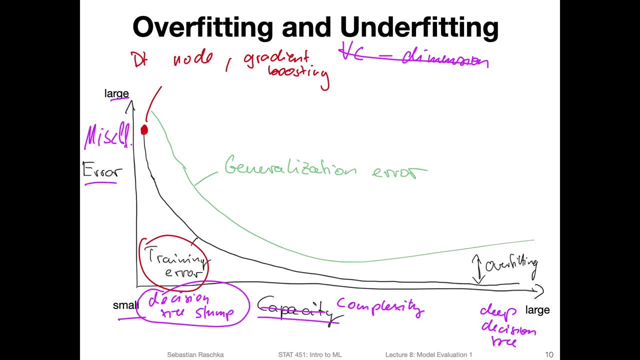 and even though overfitting is relatively small- so there's a relatively small degree of overfitting- we also have usually high test set error. So the generalization performance is also not very good, because we neither fit the training set very well, Nor do we perform well on unseen data or tested 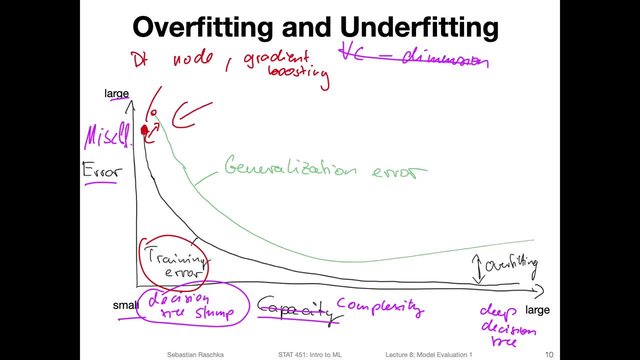 data. So here this would be a case where we under fit. So we have the problem. Merci, and I think it's it's exactly right. You said that it doesn't really perform well on either the training and the test it. So 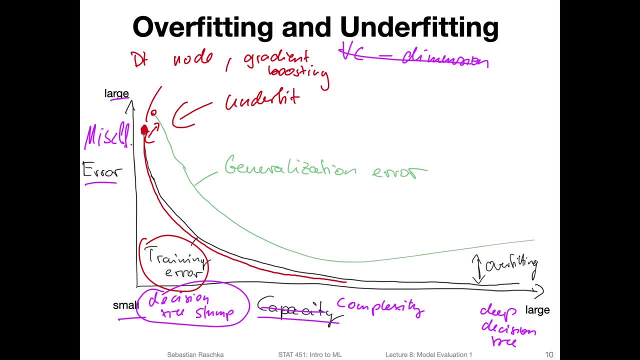 then there's a time when we make the model more complex. So if we allow the decision tree to have a larger depth, then that the training set error goes down because we fit the data set know better. And there's also a sweet spot here where we perform. 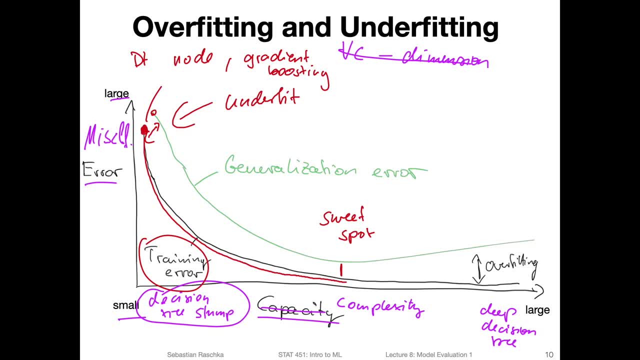 well on unseen data And on data. so on the test set on new data. Now, if we add a higher capacity to the model, if we allow the decision tree, for example, to be very, very, very deep, then it may be fits the data set way. 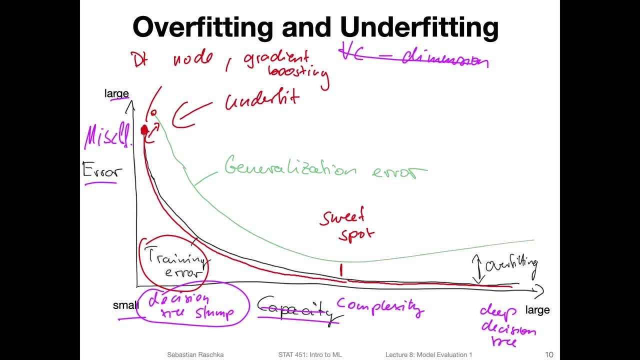 too closely. So instead of decision trees you can also think here of one nearest neighbor classifier, where here you maybe have a three nearest neighbor classifier And here you have a 13 years neighbor classifier, something like that. And if you fit the training set too closely, you will observe. 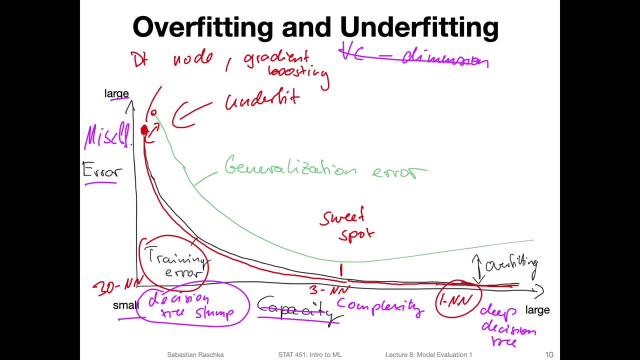 Okay, you will do very well on the training set, like for the one nearest neighbor classifier where you have a 100% training accuracy or vice versa, because we talked here about the error. we have a 0% error if we have one nearest neighbor classifier. 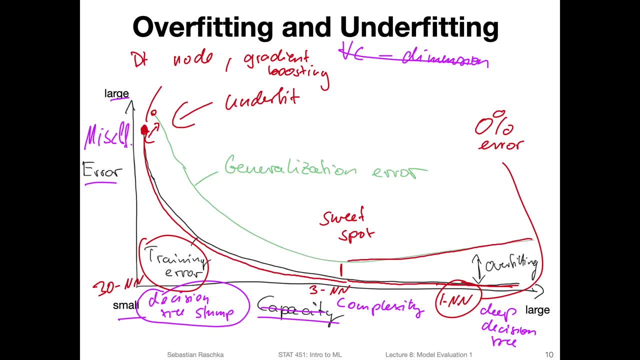 however, we will see then that we will then also start performing worse on unseen data, because now we fit data set too closely. So there's usually a trade off between the model capacity. we usually want to have an model capacity that is not too large, because then 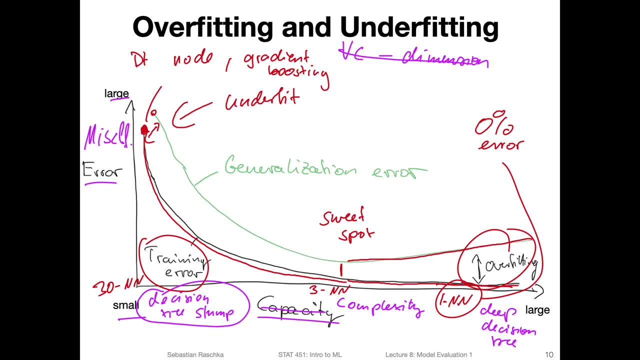 overfitting increases. But we also don't want to have a model capacity that is too small, because then we will be underfitting, which means that we neither do well on the training set data nor new data. Yeah, so sometimes in practice, also when you read research. 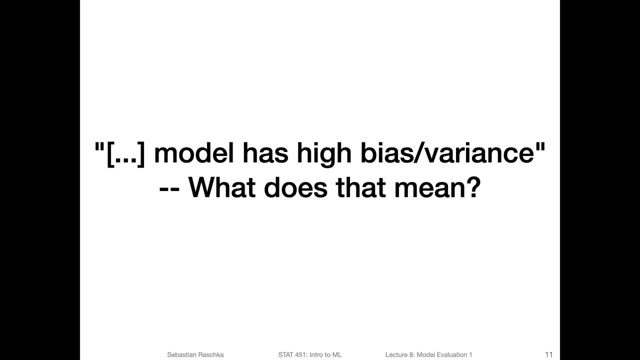 articles or textbooks or blog posts on the internet. what people often talk about is that a model has a high bias or high variance. Instead of talking about overfitting and underfitting, people just sometimes use the terms high bias and high variance. So what? 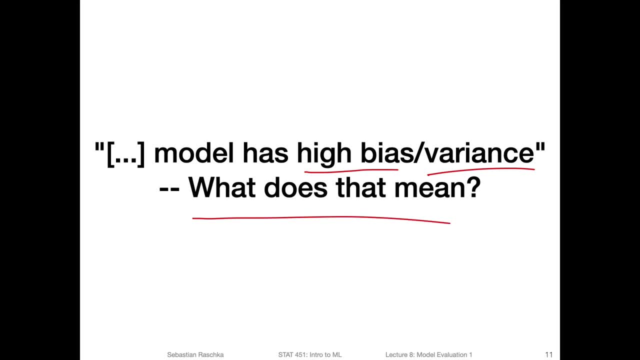 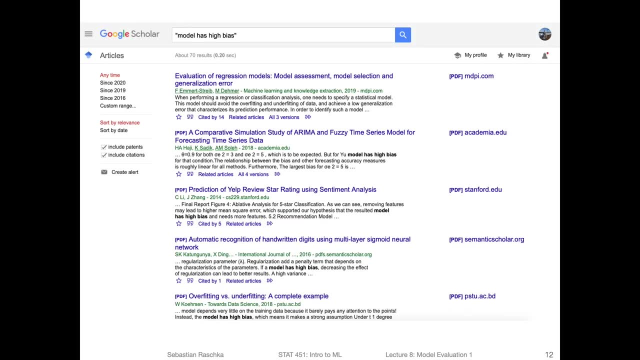 what does that mean? What does high bias and high variance mean? So in this lecture we'll also talk about how what that means and how that's related to overfitting, underfitting. So yeah, just as an example, when I type model has high bias into 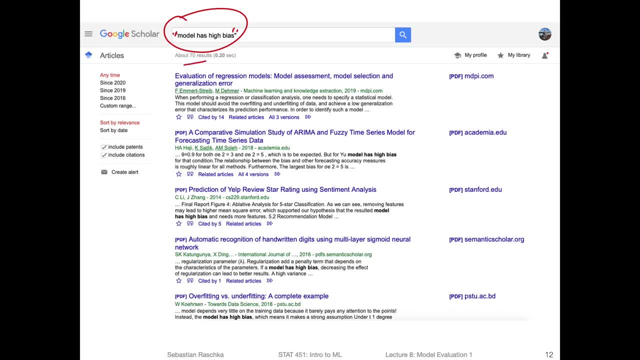 Google scholar. if I put this verbatim, there are actually even 70 hits here people saying the model has high bias. that's actually not uncommon in machine learning on different flavors of phrasing that. So here I was just searching verbatim, But yeah. 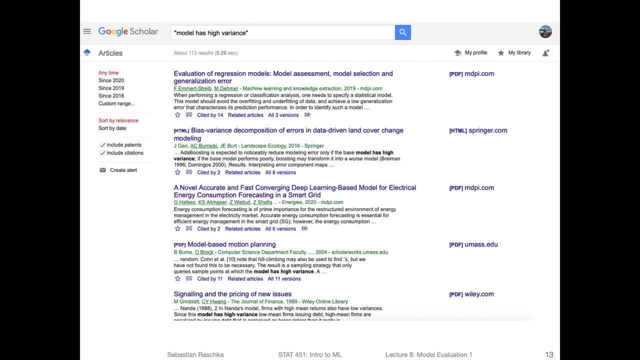 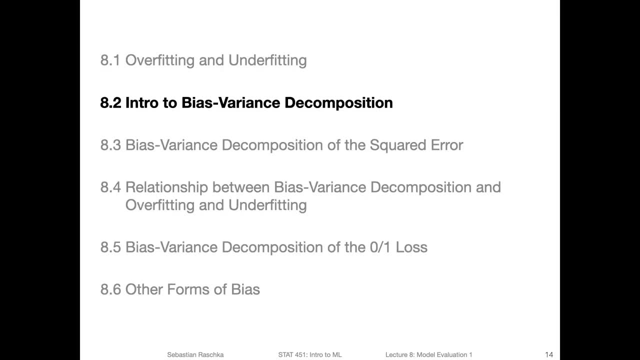 it's often the case that people say a model has high bias and equivalently high variance, instead of saying the model overfits or underfits. So what does that mean? And that is something we will discuss in the next video.